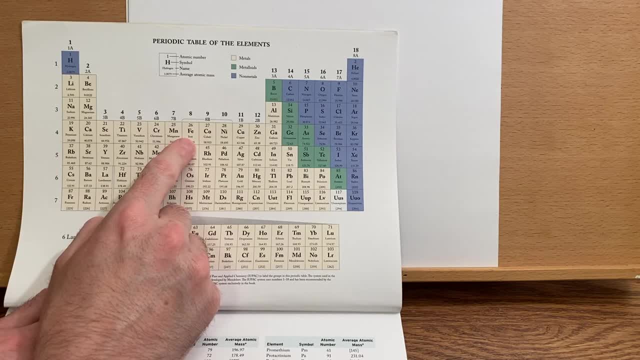 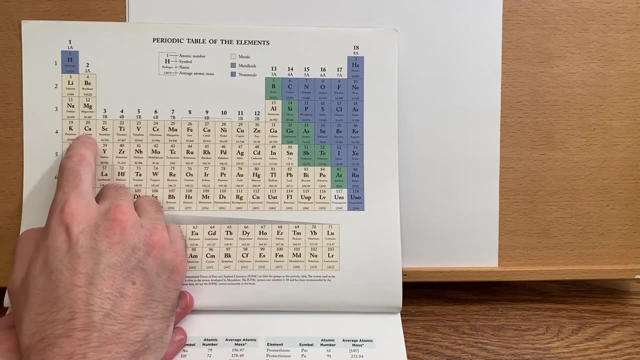 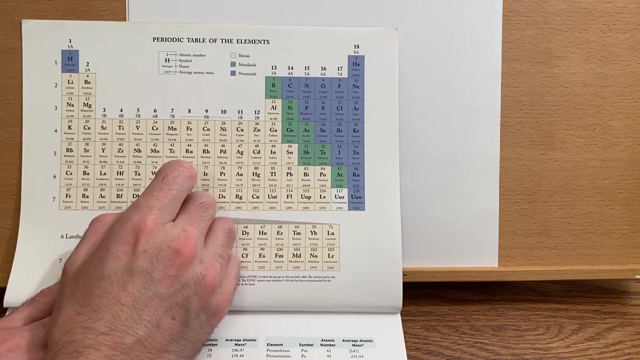 3d6 electrons. So this is a d6 ion. Now, if we went to iron 3 plus, we would lose the two 4s electrons And one 3d electron, which would bring our configuration to 3d5.. Went from 6 down to 5. 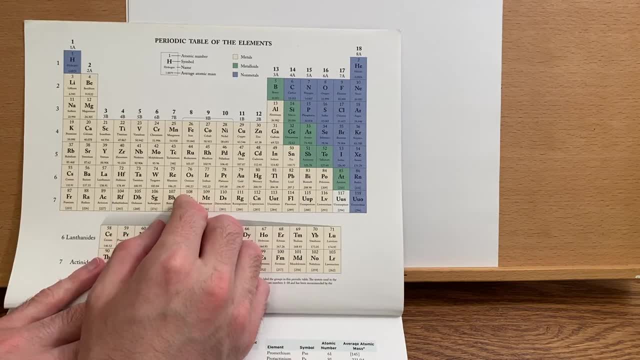 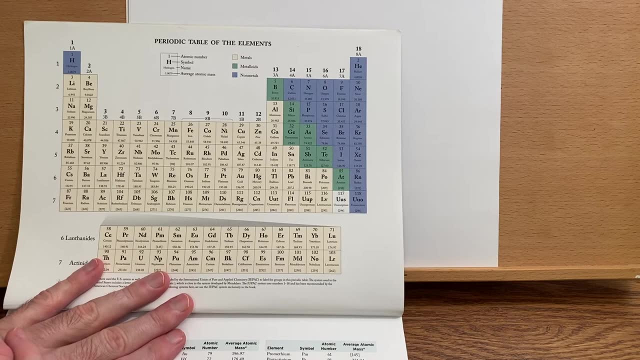 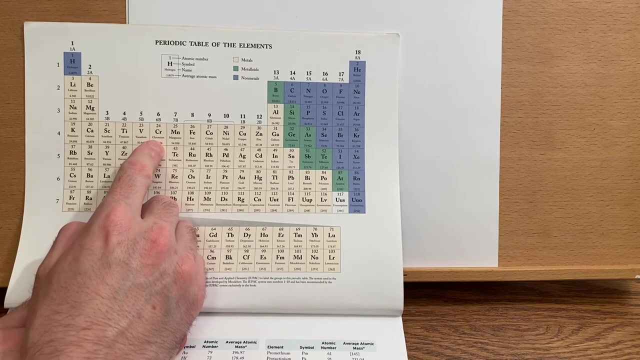 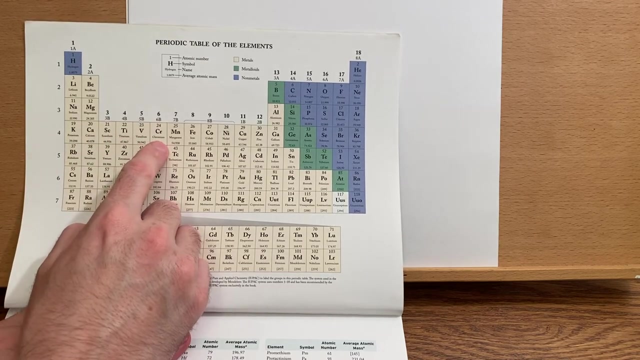 because we had to lose one d electron. So let's just keep that in mind when we're determining the electron configurations of these. Now you might say, oh, remember, there's those exemptions or exceptions. Chromium has 4s1, 3d5. And to that I say: well, most of the time when we're dealing with 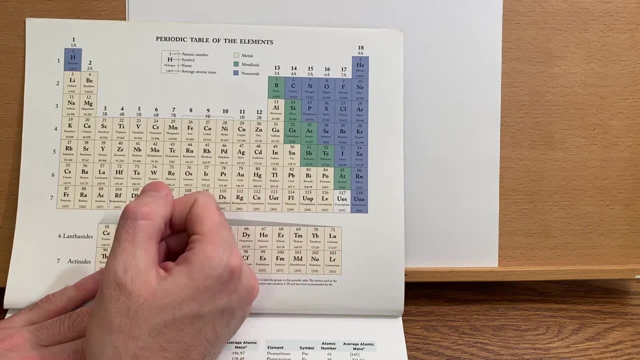 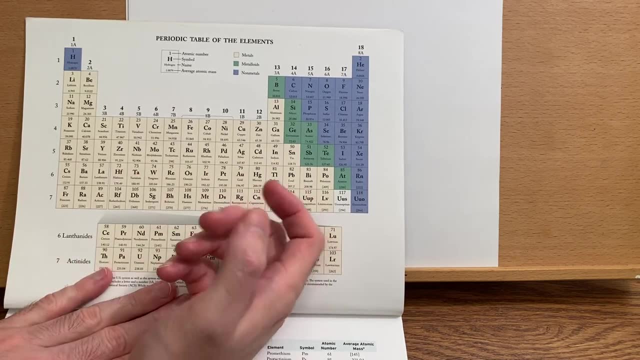 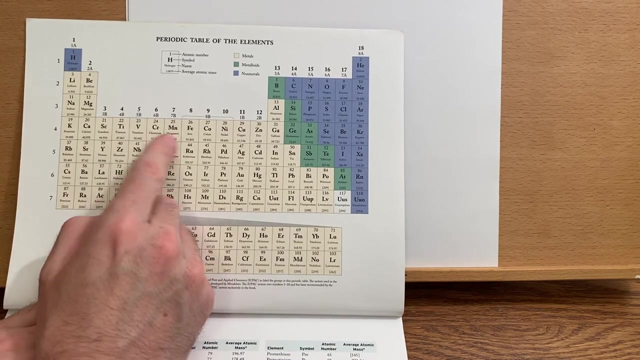 transition metal complexes, we have either a plus 2 or a plus 3 charge on the metal. That's the oxidation state, And since we take away the 4s electrons first anyway, and generally the transition metal element is going to be less than 2, then we're going to have a plus 2 or a plus 3 charge on the metal. 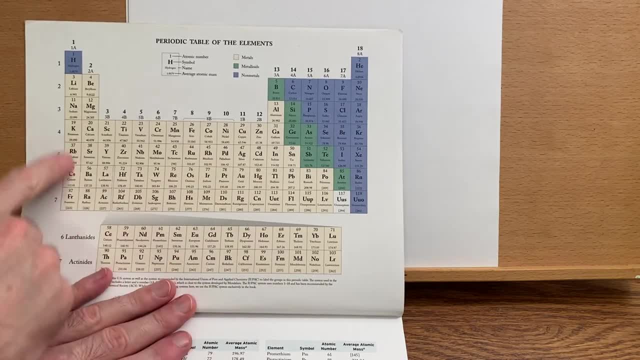 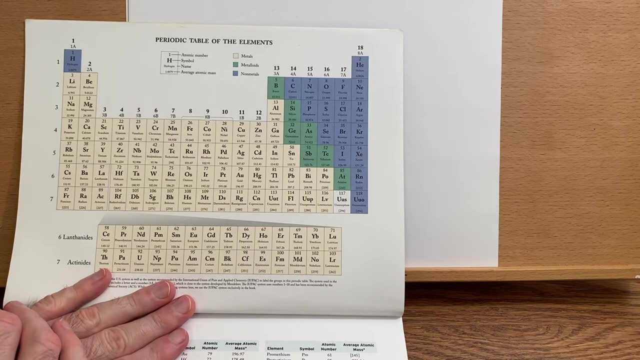 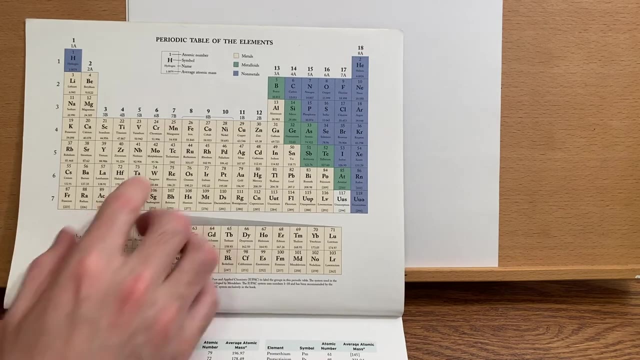 are plus 2 or plus 3, these 4s electrons are gone anyway, so it doesn't really matter. In fact, there are quite a few other exceptions on the chart, and there's enough that I don't actually remember all of them. I do know that the chromium is 1 and copper is 1, but again,